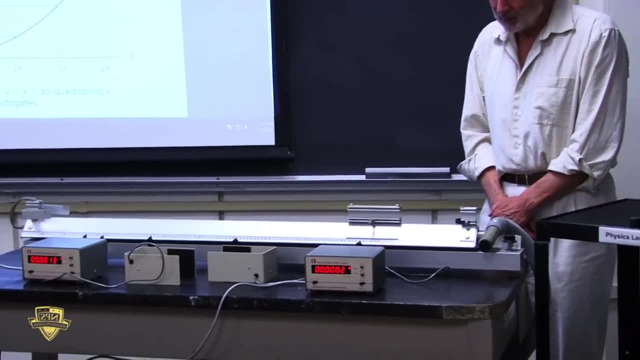 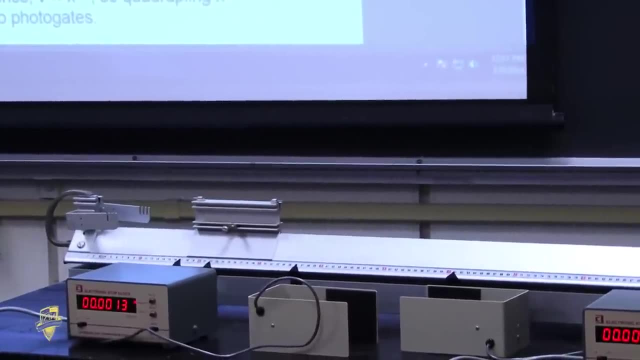 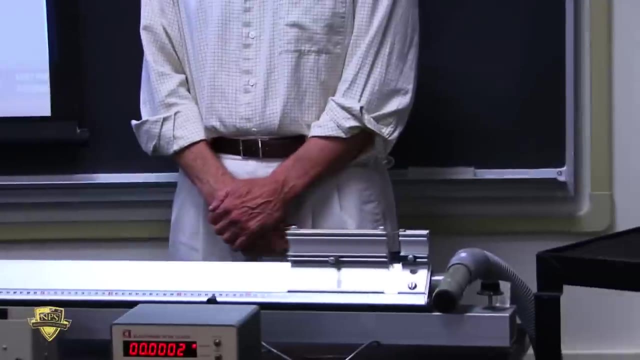 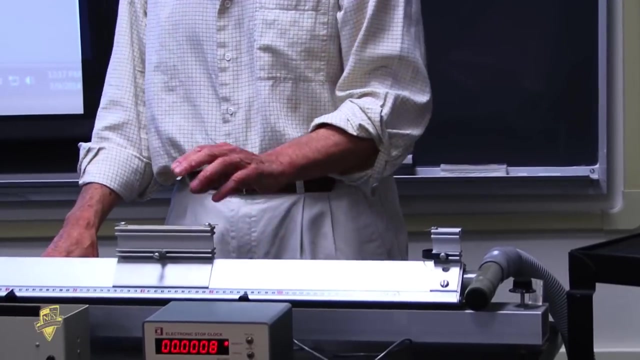 It's pretty level. Let's check it over here. Yeah, Not quite level, That's going to move. So what if I give it some initial velocity? How would you describe the motion? The motion you just saw there, Pretty constant velocity. 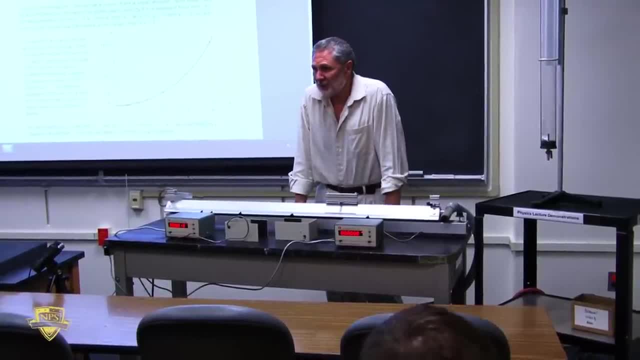 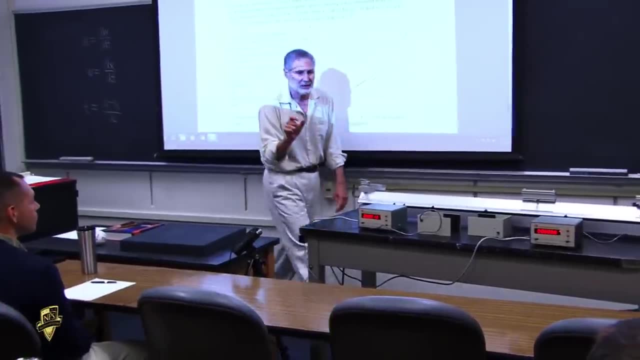 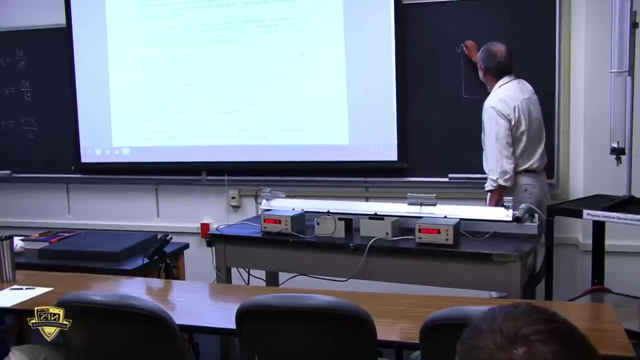 I'm sorry. Constant velocity- Yes, It looks constant. The rate of change of position with respect to time is a constant, So over any time interval it always covers the same distance. That's constant velocity. To beat it to death, here's another way. 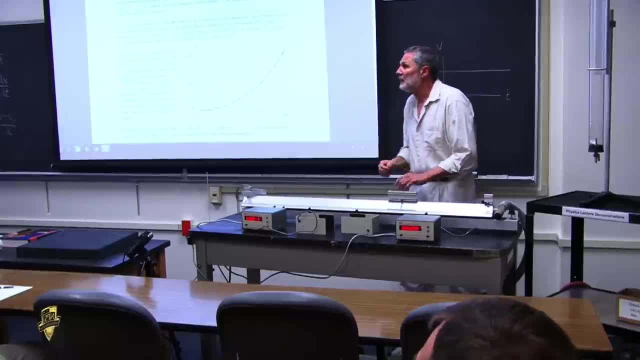 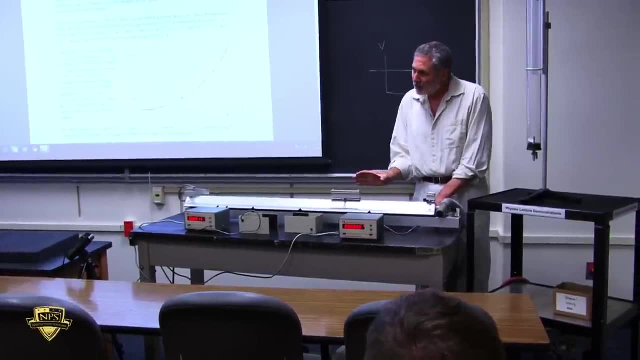 Constant velocity, Except when it collides and bounces back. Yeah, Now that's getting ahead of the. It's unavoidable here. What's going to happen when it bounces back? It comes in with a certain speed. Speed is the absolute value of velocity. 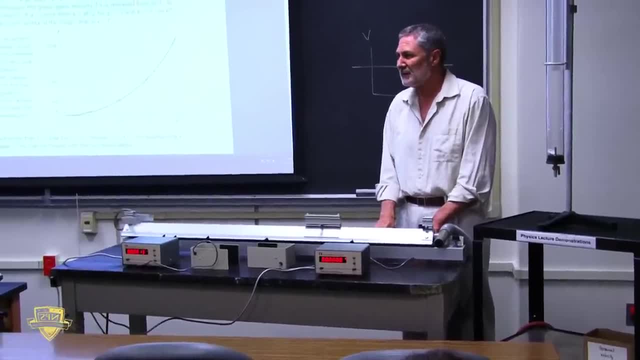 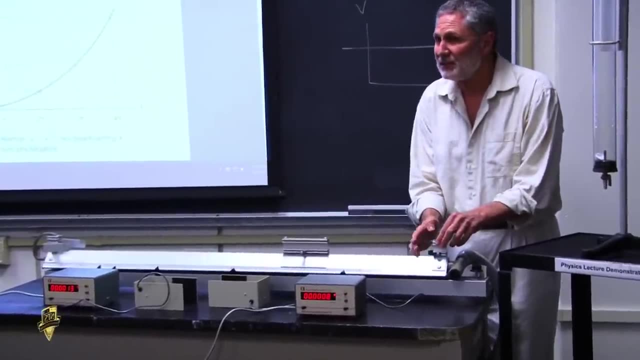 It goes out with. What's the speed you think it's going to go out at? Almost the same. Yeah, This is a fairly pretty good elastic. This is nearly an elastic collision. We'll go through all this when we get into collisions. 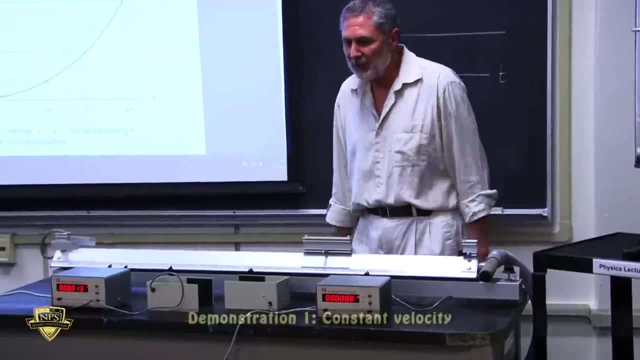 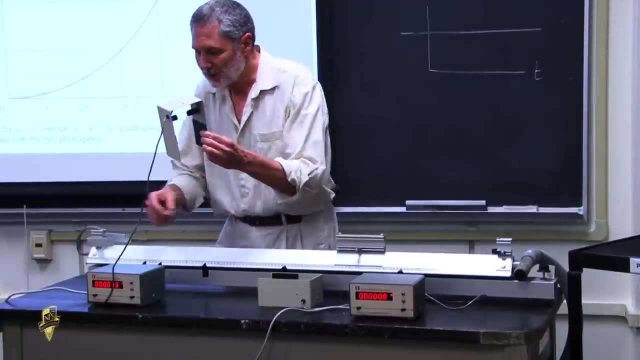 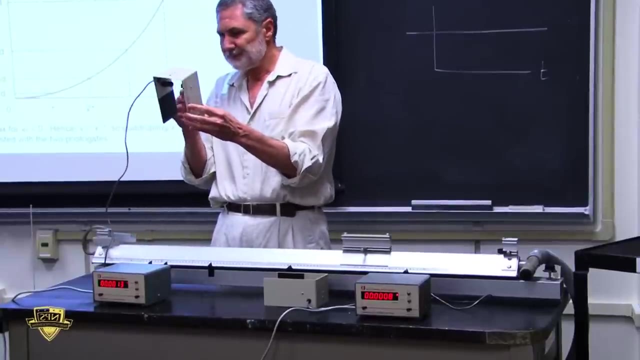 But you can kind of see that it does that. Now we can test, We can quantify how constant the velocity is with these photogates. here We'll be using a similar apparatus in the lab. Okay, So one of these, I don't know which, is an infrared light source. 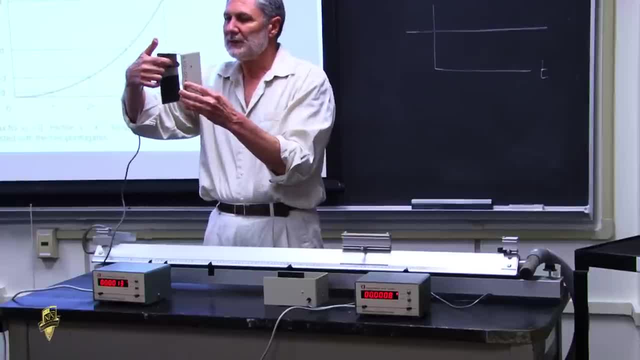 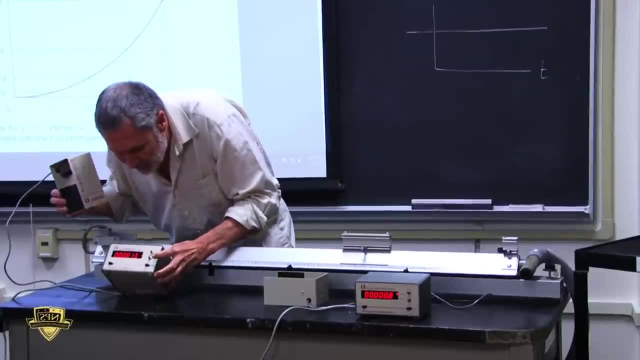 It sends out a beam, Let's say this one. It sends out a beam to here And here there's a photo cell that picks up on the light. And what this box right here does- Let me reset it- Is when you interrupt the beam, it starts a timer. 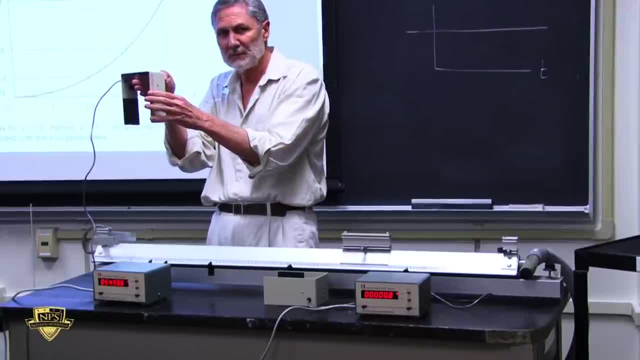 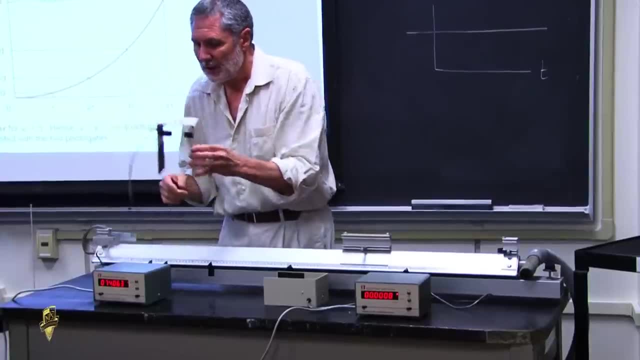 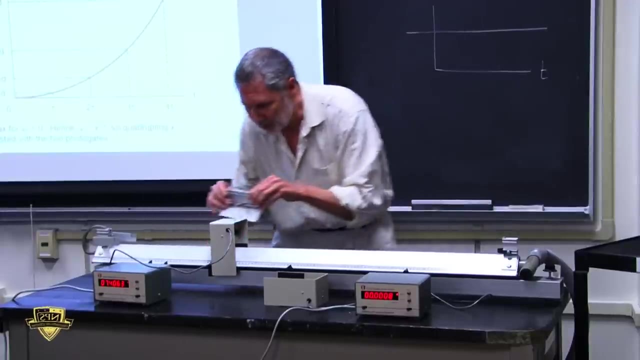 It should be going Good Because we've had trouble. And then when I stop the beam, when I restore the beam, it should stop. So we can utilize this. We can put this at some point here. Here's the glider. 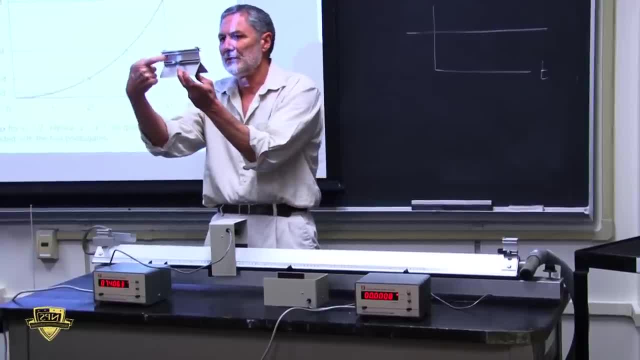 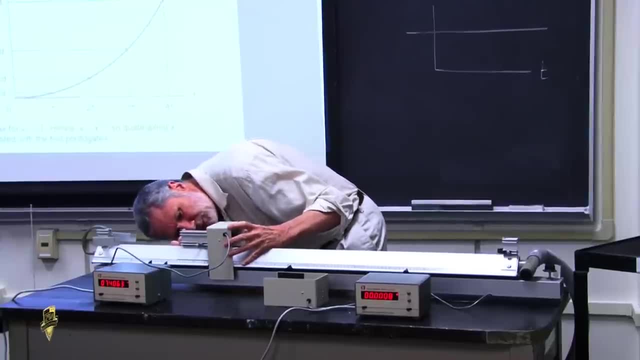 Now I'm going to have the glider. This looks kind of ugly. I'm going to have it interrupt this distance Of the glider. When the glider moves by here, it's going to interrupt the beam. Okay, And I'm going to do the same thing here. 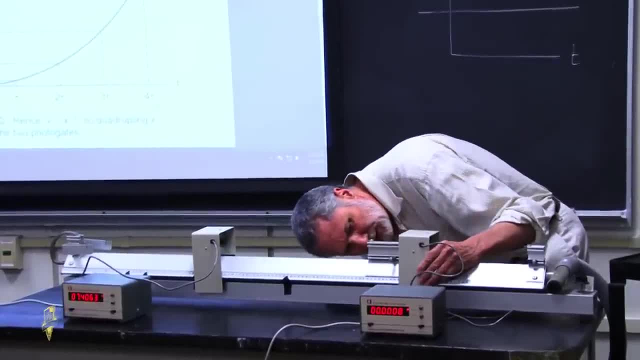 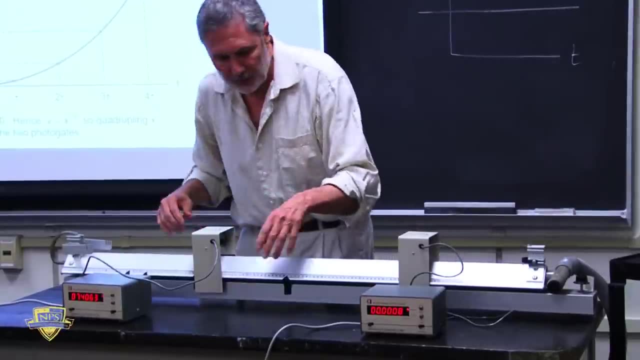 I need to. I'm adjusting the height right now. Okay, This. This shouldn't work. Okay, Now I want to. Is this working, Gosh Sometimes? Okay, Hopefully, this one will work. Okay, Now I want to. 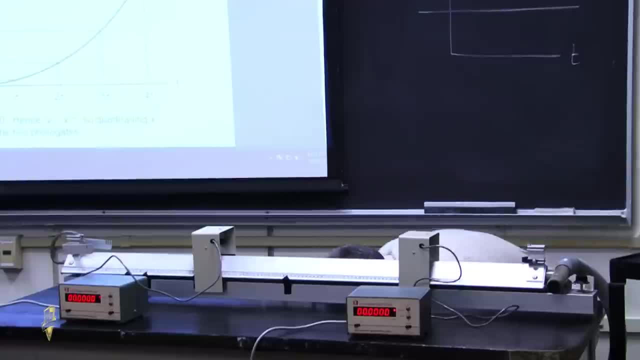 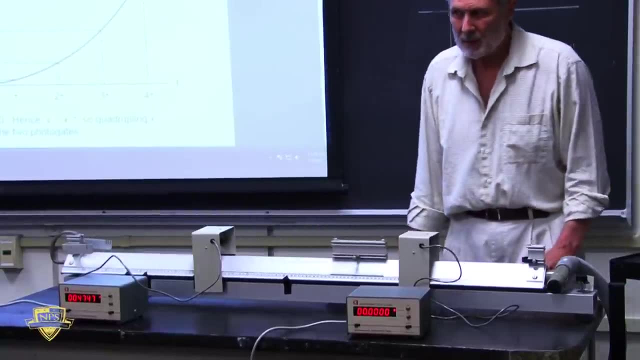 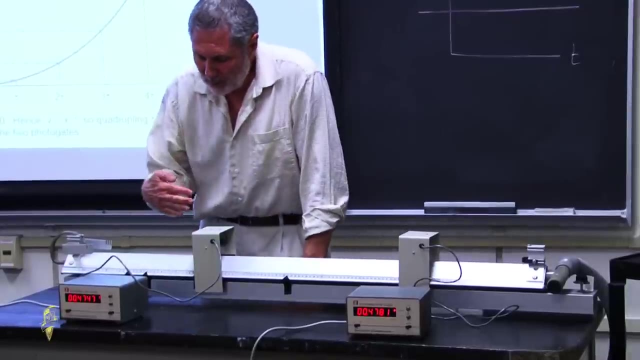 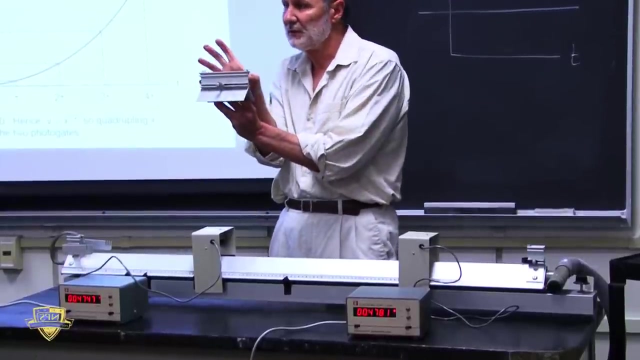 Is this working Sometimes? Okay, Hopefully this one will work. Okay, So If we know the time this is interrupting and we measure this distance, we can get the velocity, Actually the average velocity. We will take this distance divided by that time and that's going to tell us the velocity. 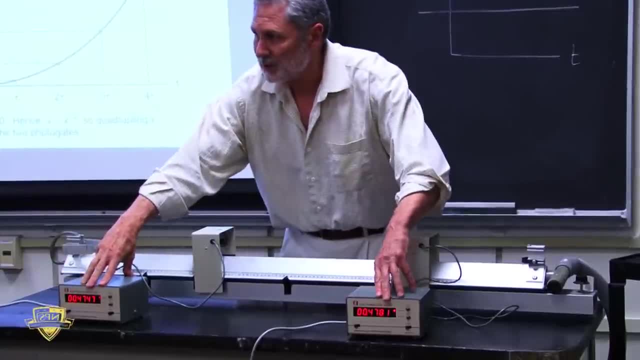 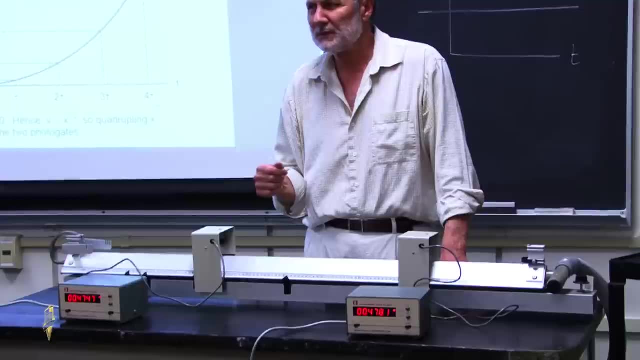 The average velocity. Now, these two times should be pretty near each other, Really, Yeah, Okay, This time should be What? should it be A little bit bigger than this time or a little bit less? It should be a little bit bigger because it's probably 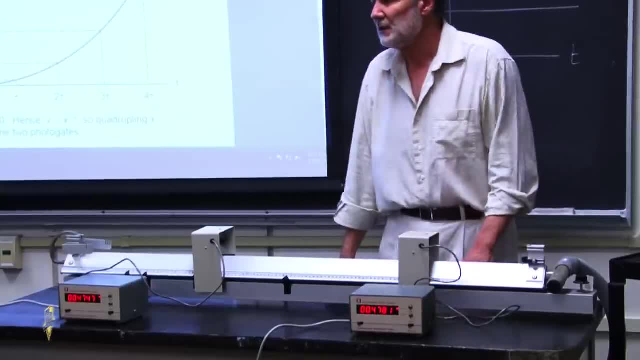 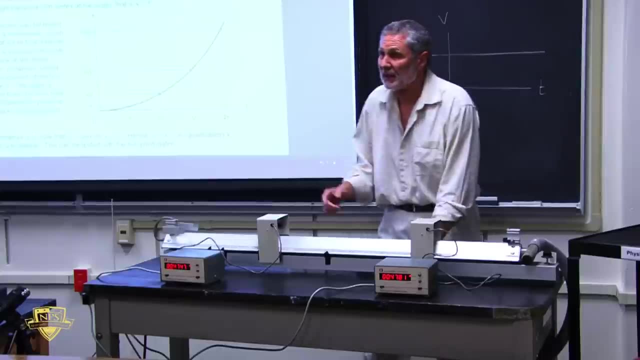 Is it? Yeah, Okay, Yeah, I'll believe you. I believe you. I tested this and I'm sick of this. Okay, All right, So we'll be using this kind of This is common in mechanics labs to use this. 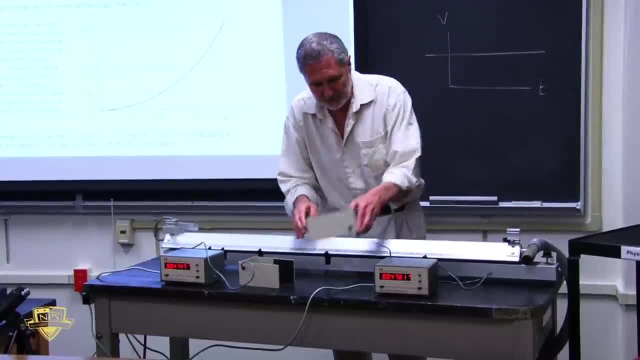 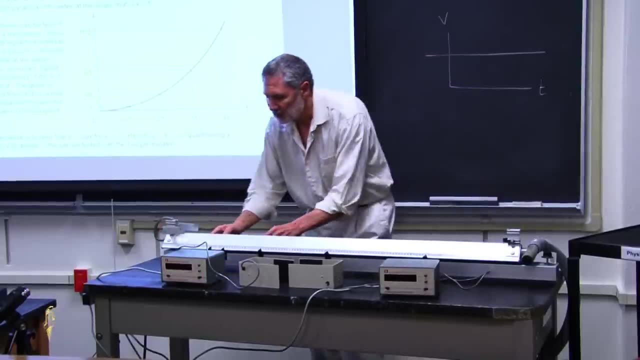 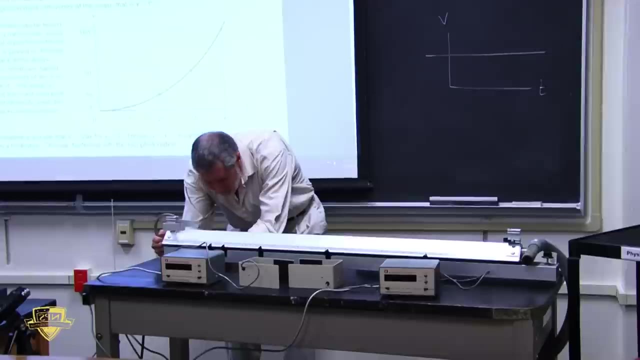 The next thing we're going to do: Get rid of these. I guess we can turn these off, Okay, All right, So Okay, The timer's off. The timer's off Now. this is an anodized aluminum plate. 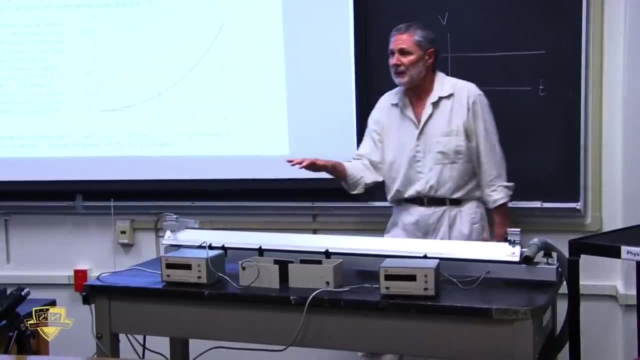 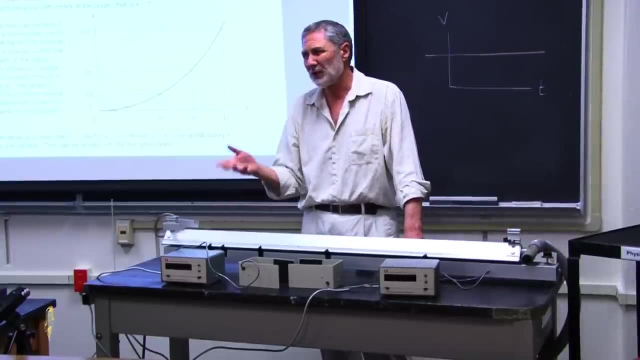 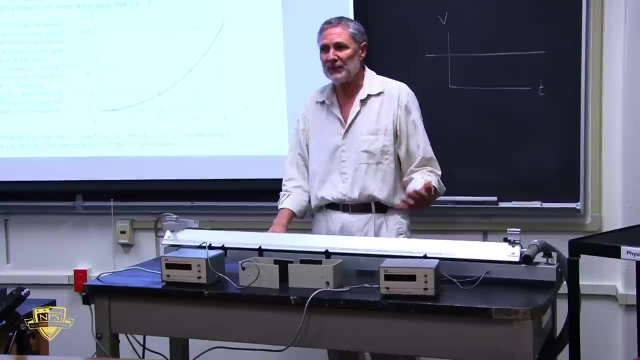 Now we have what's called an inclined plane. Okay, And this is one of the things that Galileo investigated. Now Galileo used rolling. We'll talk more about this when we get to dynamics. What he was doing was he was really interested mainly in freefall, but it just happened too. 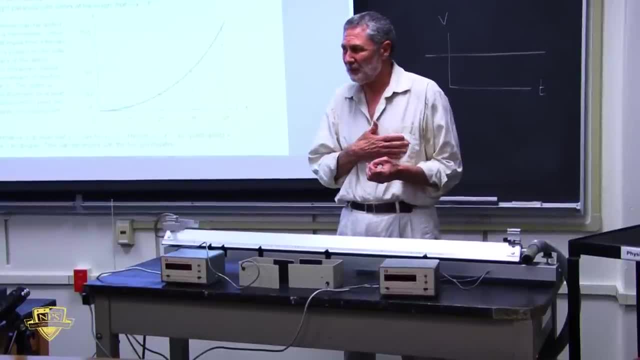 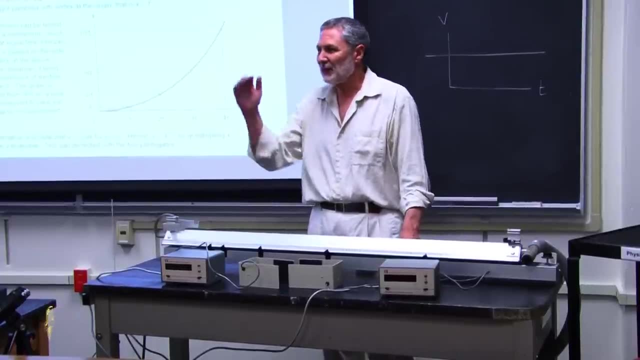 fast. You know when your timing device is like your heartbeat or an hourglass. that's- I'm not kidding- Okay That you Freefall is just way too fast. So he recognized that if he had an inclined, If he had a plane that's inclined, that it should be essentially like gravity, but it'll. 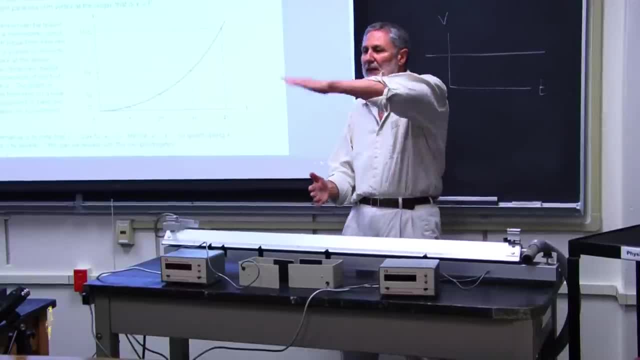 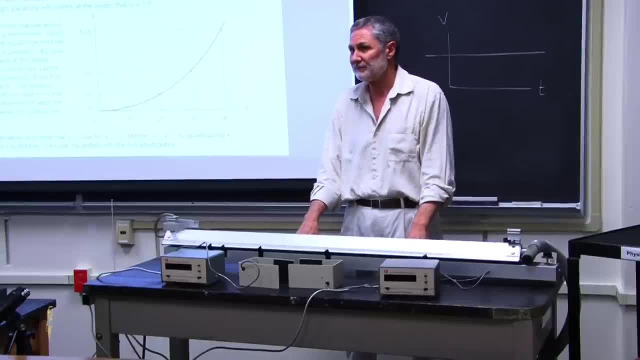 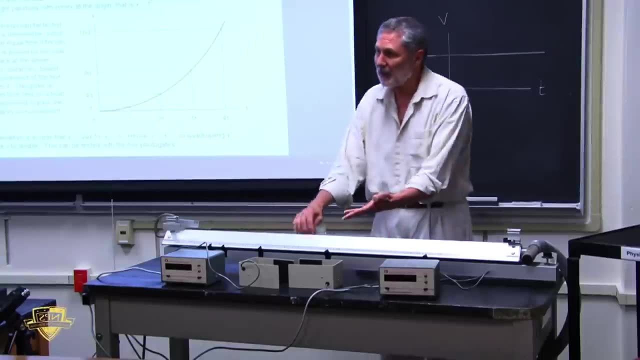 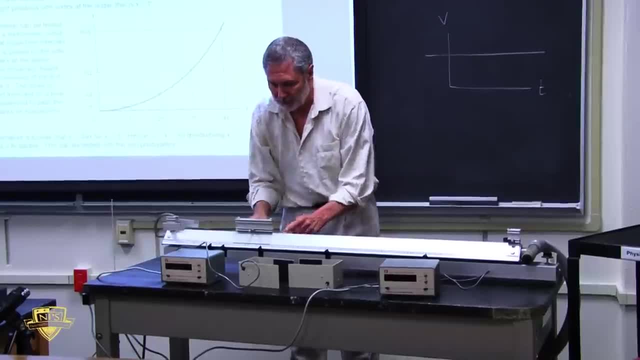 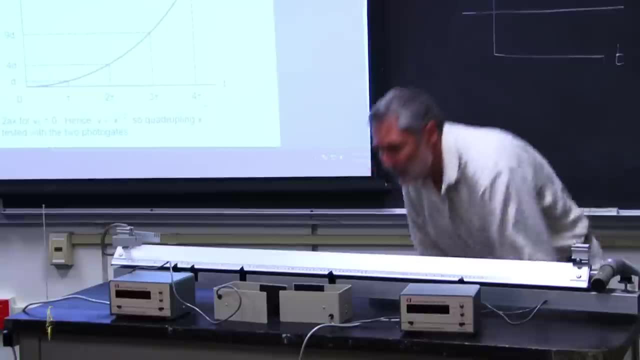 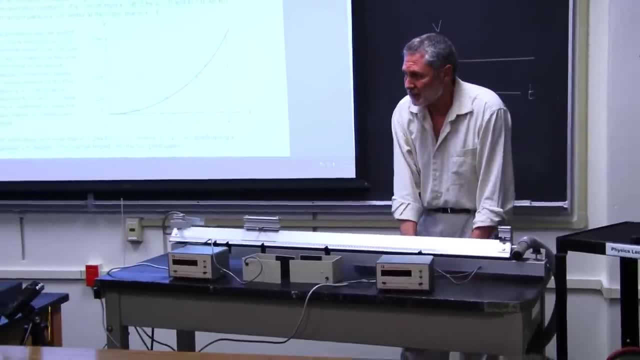 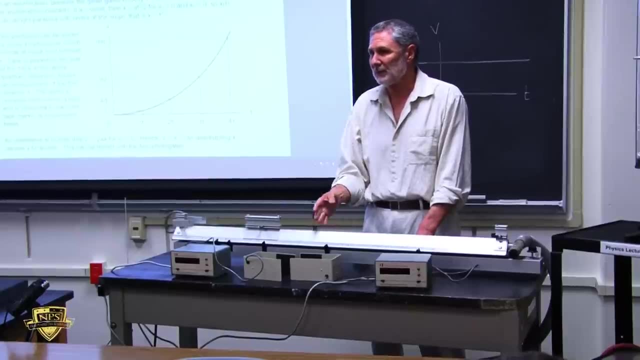 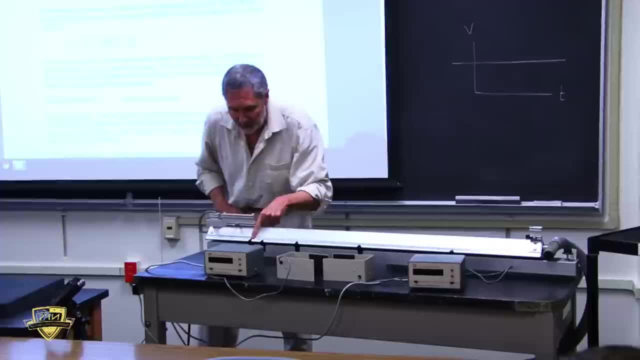 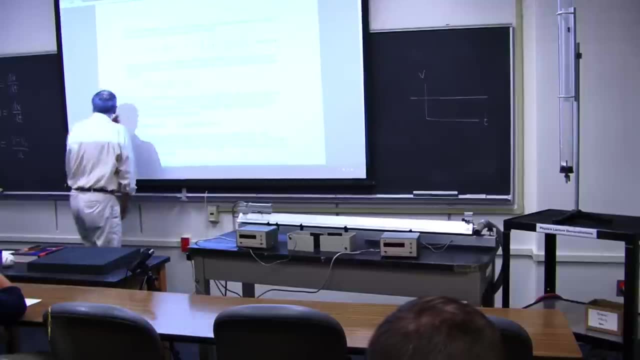 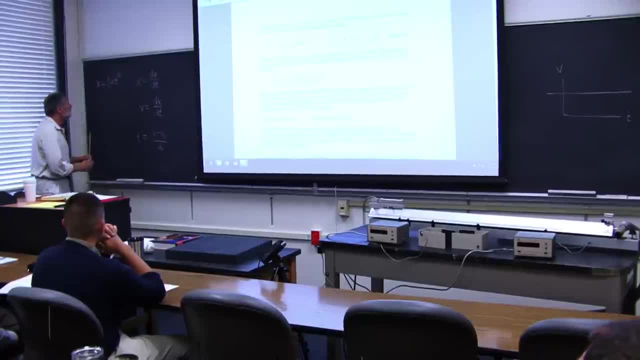 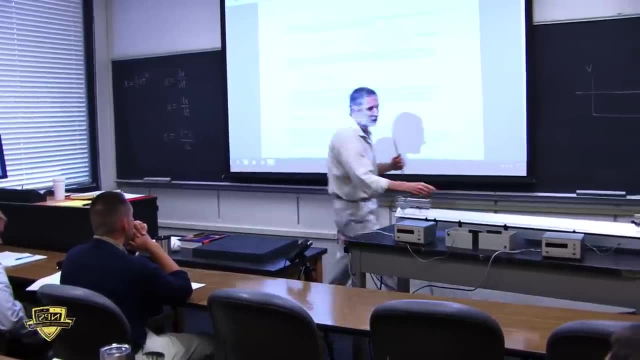 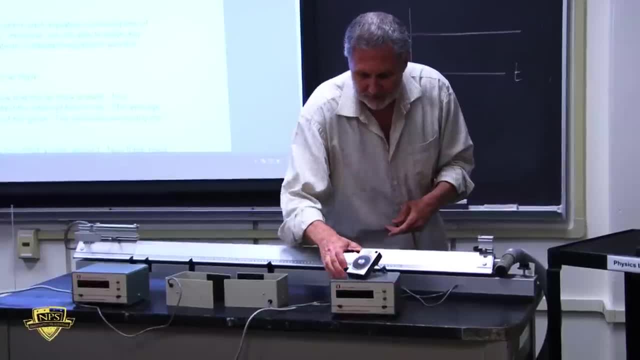 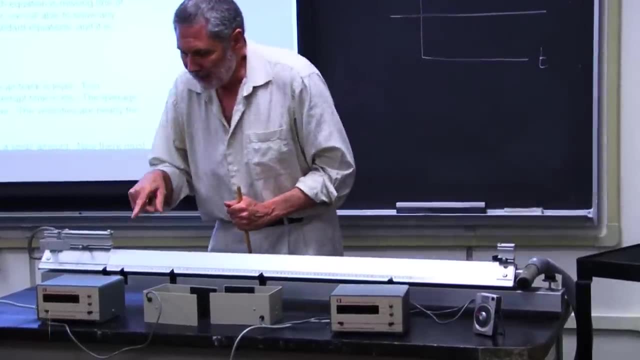 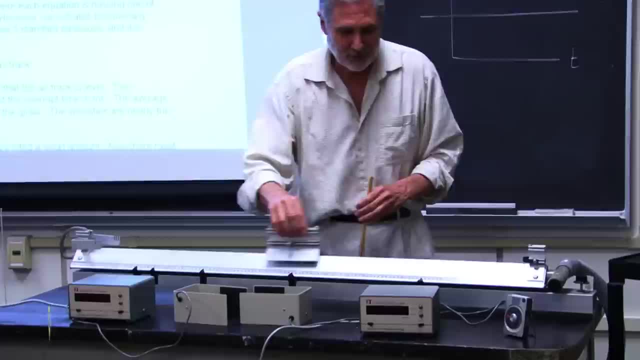 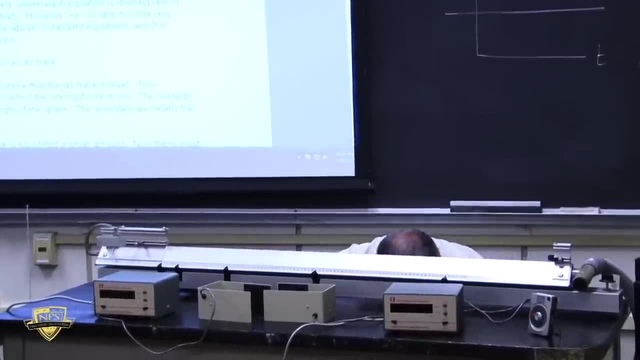 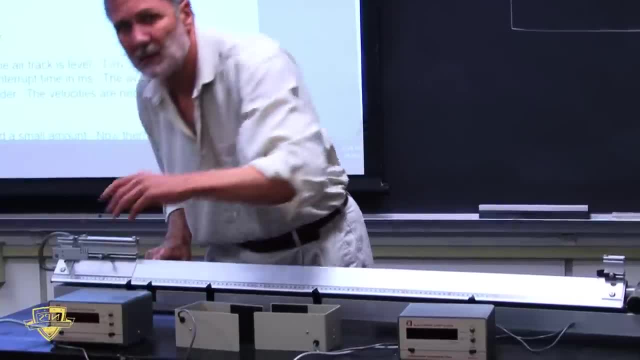 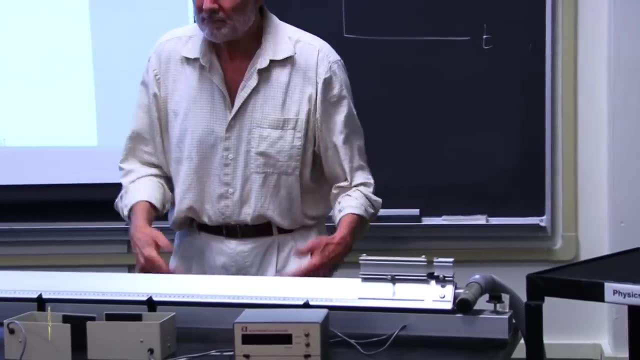 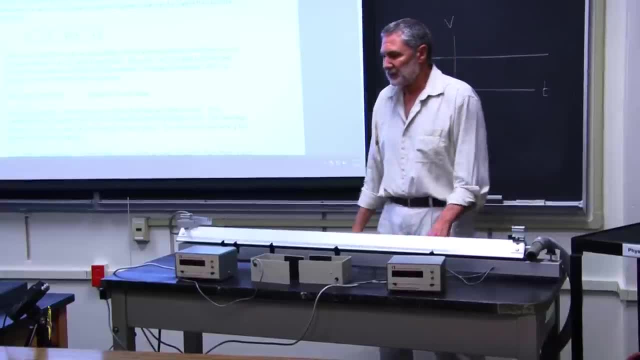 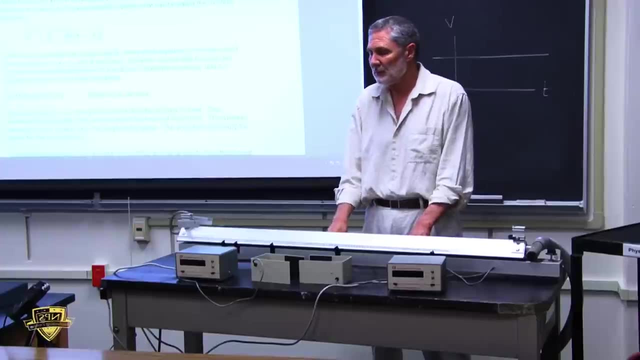 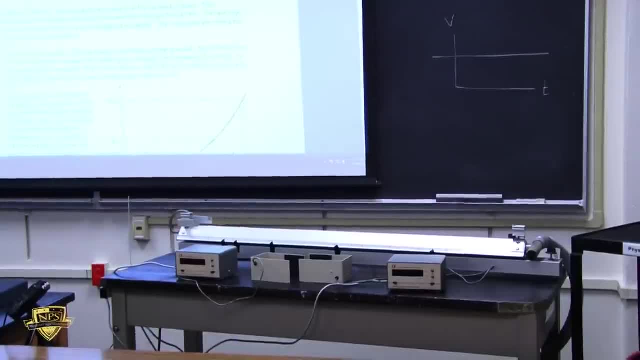 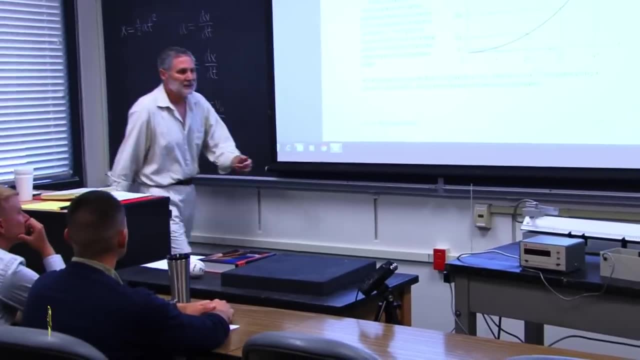 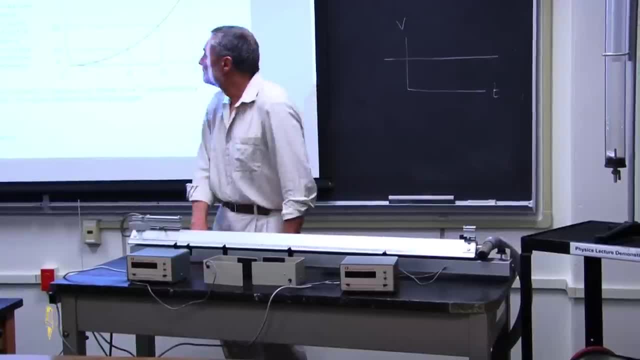 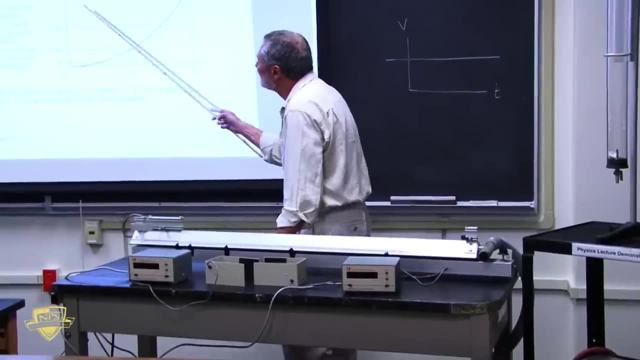 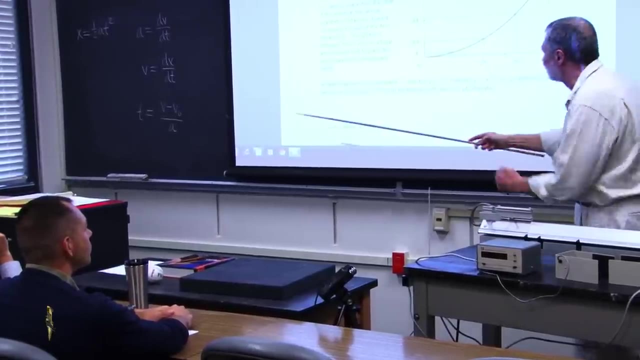 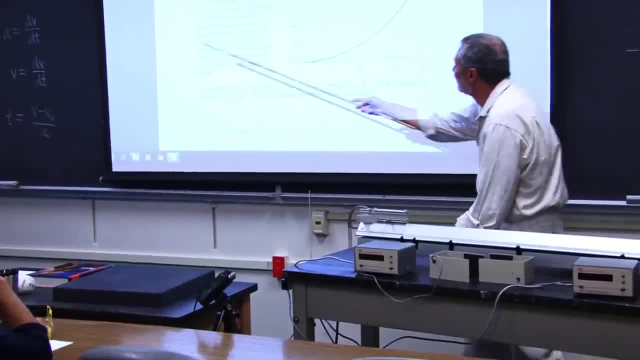 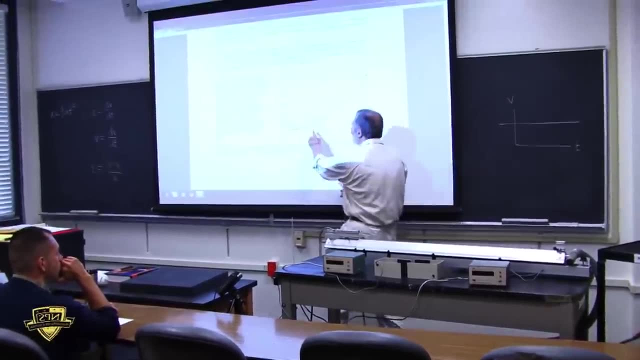 at the bottom of the parabola, right there. So this is a sketch of what that looks like. And if we sample it at equal time intervals, which is what the metronome is doing, right, you can see that the displacement 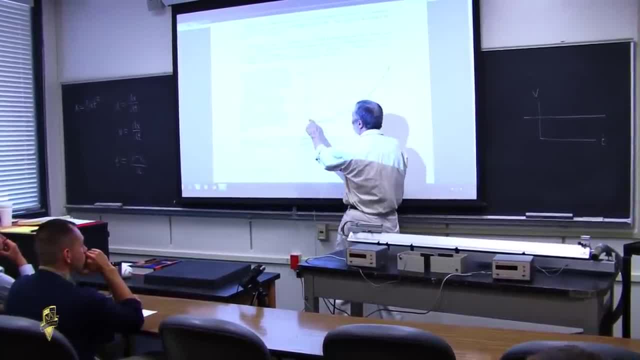 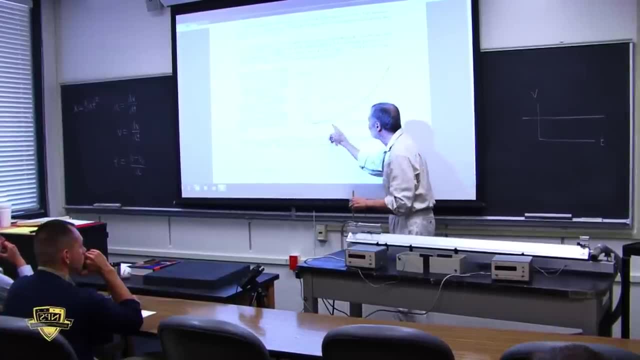 there will be some value here. Here, because of the square, it's going to be four times. Here it will be, you know, two squared, Here it will be three squared and four squared. So what you just saw there in the demonstration was 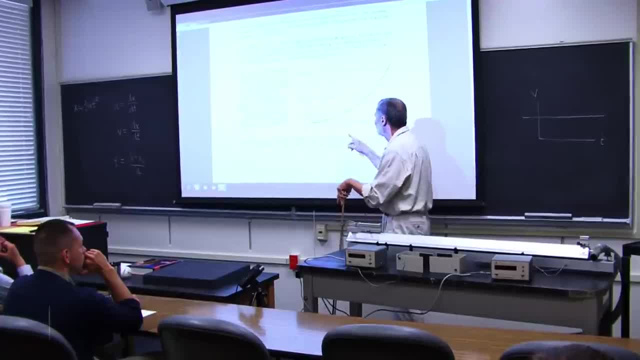 if you observed where the glider is when you hear the metronome, it's at these points, right. I started here. tick, tick, tick, tick, tick and it was right where the I placed the tape according to that. 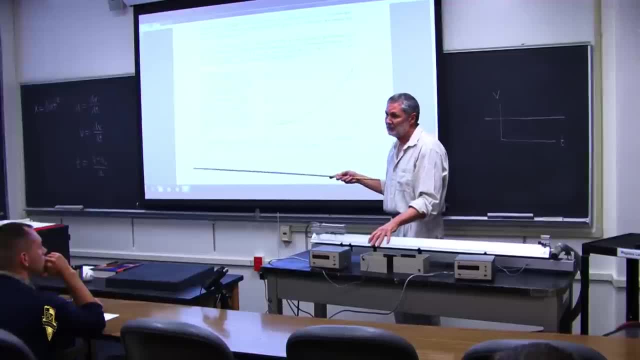 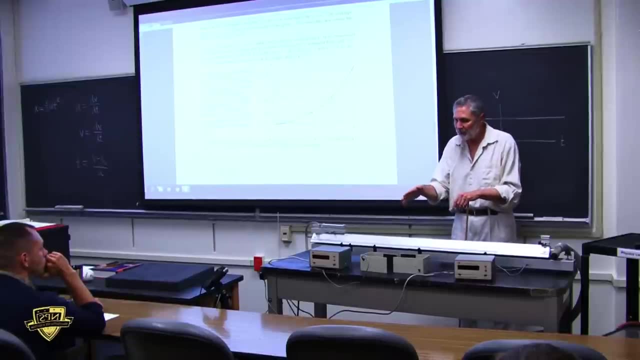 Now, you know, for me to do this, I needed to know the acceleration, And we're going to develop, we're going to develop a formula for it. It's simple, with the acceleration, here We're going to in dynamics, we will. 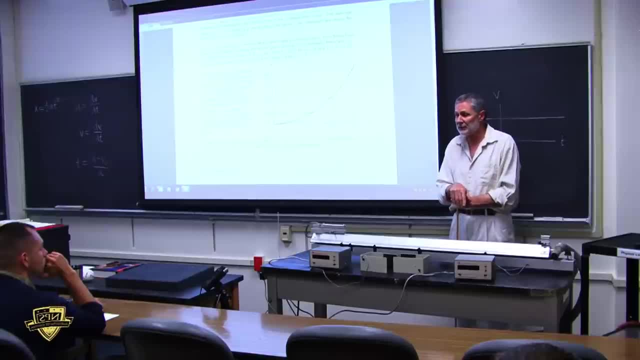 it's one of the first systems we're going to look at. We will show that the acceleration is constant And we'll come up with a formula for what the acceleration is. I had to do that, to do this And suddenly you see this thing: this is sloped right.